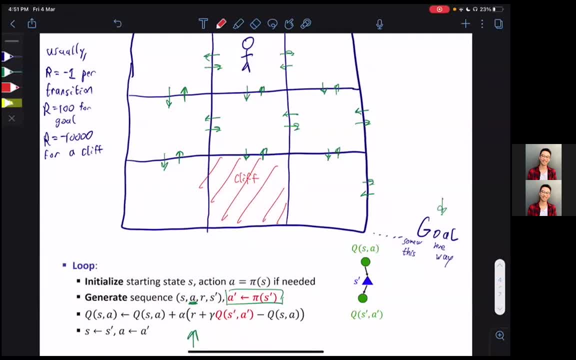 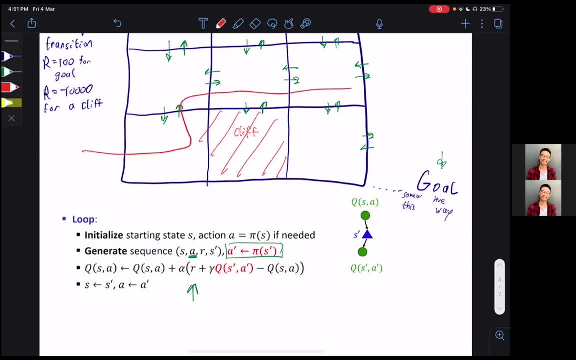 way it generates these paths right is by calculating different Q values. right: Calculating different Q values and finding the best Q values that give a path that will go around the cliff, something like this right, Where the cliff is just like an area with really, really poor. 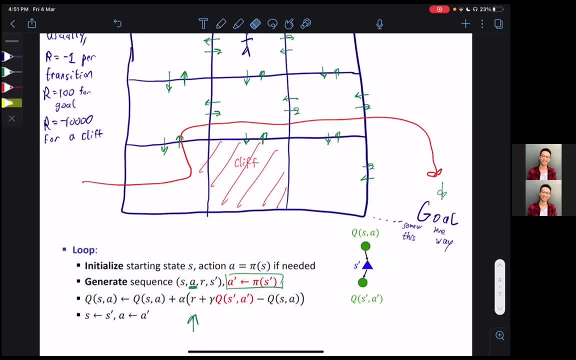 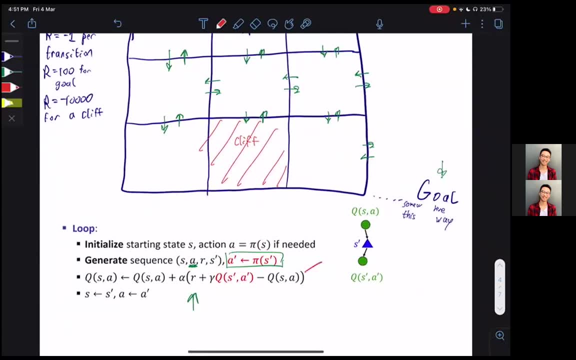 reward, So you always want to avoid that. The key thing to notice about the differences between these two algorithms is that pretty much the way you generate your successor states or successor action and the way you calculate and update your current state action pair right These algorithms. 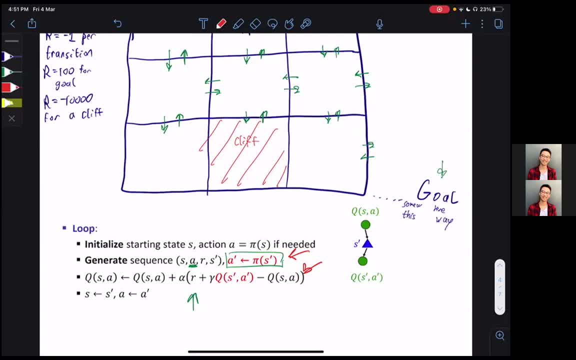 give quite different outputs, but the way you actually implement them are very, very similar. Like they're, the differences are quite subtle, but the outputs are very different And today I'll be just doing my best to go over the differences and just to explain why. I guess people like to say Q-learning. 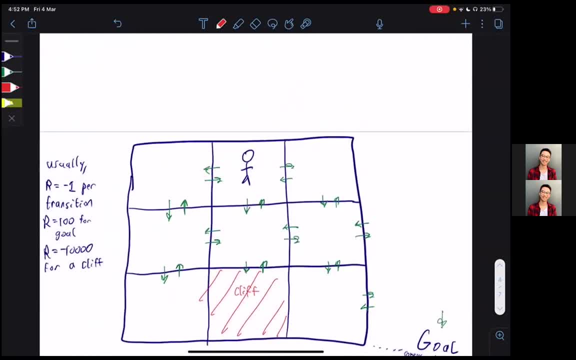 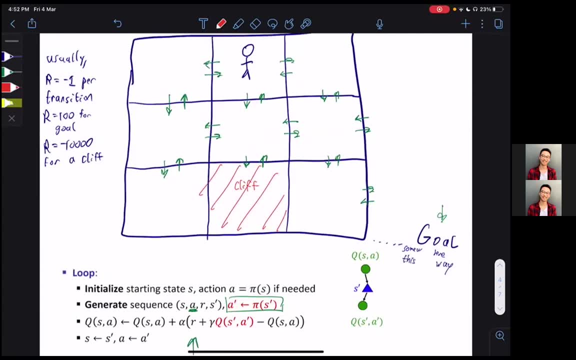 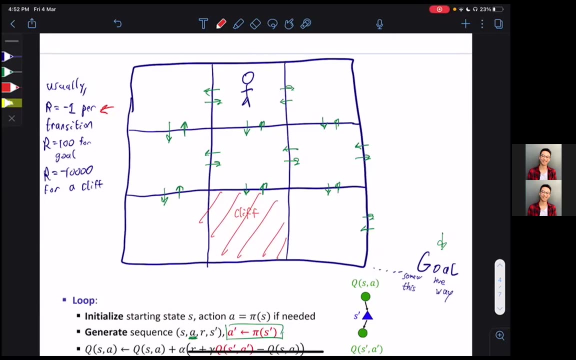 is more of like a kind of greedy optimistic algorithm, and SARSA is more, I guess, conservative and I guess accounts for more factors that go on. Just do, I guess, define some terms here. This means that for every transition action I have a minus one reward. So this: 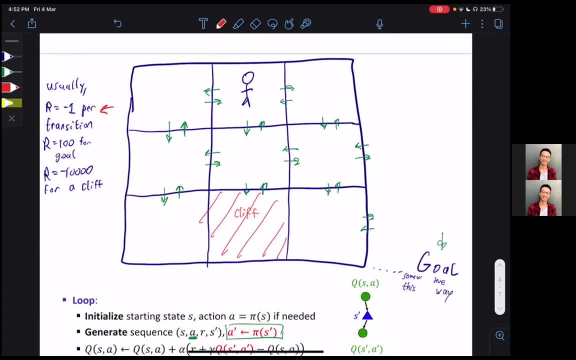 tells the robot that you know it wants to get to the goal as soon as possible, because as soon as long as it's alive, or as long as it stays alive inside this grid world, it loses energy or loses rewards. If it gets to the goal, it has a hundred reward, And and then if it falls up, 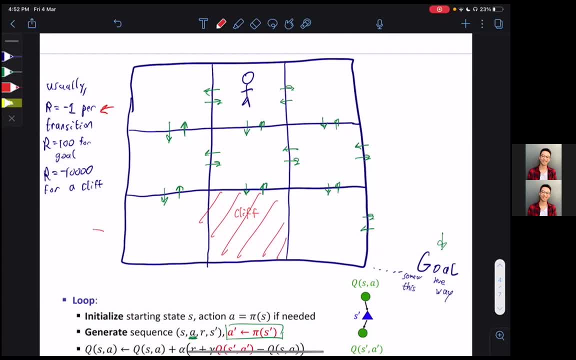 it gets to the cliff over here as a really bad reward. So in general it wants to make a path that gets to over here as fast and also as safe as possible, But depending on you know whether you're doing SARSA and Q-learning right through your algorithms. 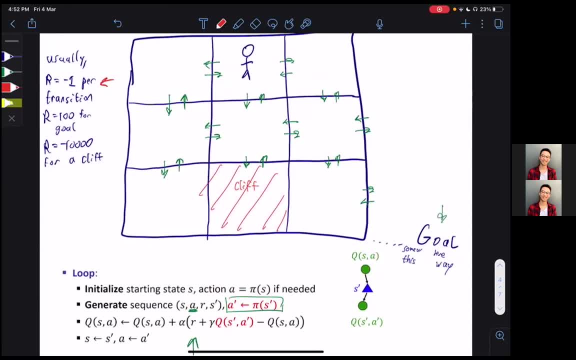 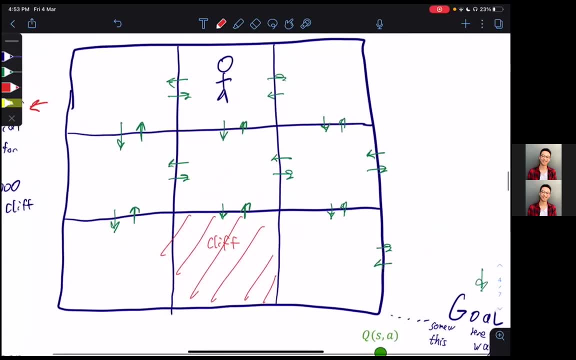 some paths might be more optimal, some paths might be more safe, and you'll see what I mean in a moment. First, I'll be talking about SARSA, So let's think about what's going on over here. So look at all these green arrows right. All of these green arrows represent your different state. 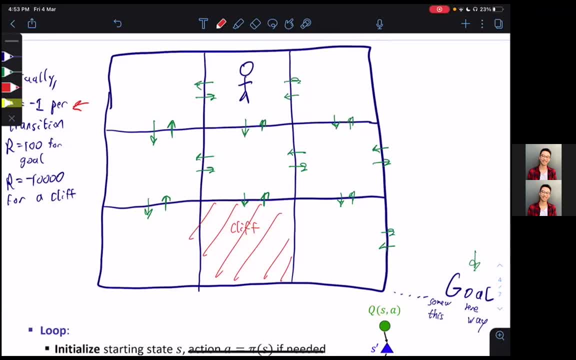 action pairs. I know I didn't draw all the green arrows possible, but just bear with me here. These state action pairs, let's say that they all have some QSA values, or values, or utility values assigned to them from before right. Right now we're in the middle of running SARSA. We're in 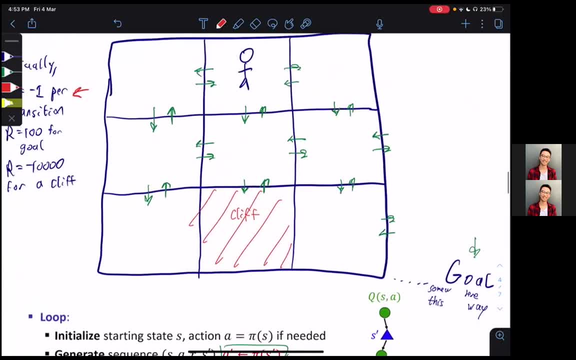 the middle of running a SARSA and our goal is to update these little- I guess- QSA values, all these little green arrows. they have numbers attached to them. Our goal is to update all these little green numbers over here so that they converge to a more optimal, they converge to a state where we can be. 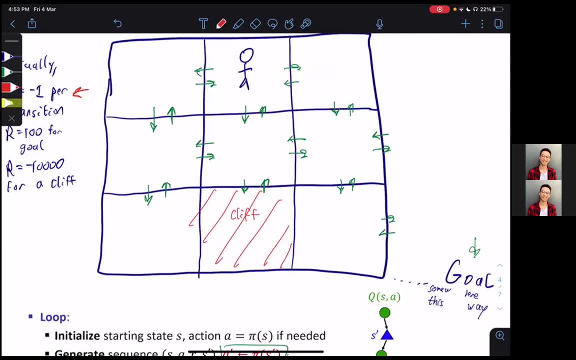 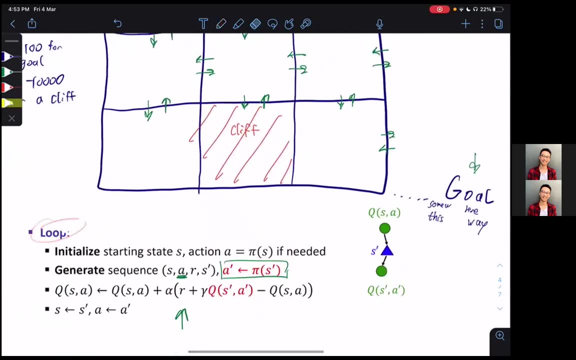 comfortably say: okay, this is what we want, And then those QSA values- the max of each state- will give us some path. that will probably look like something like this: okay, So our goal is to update all these utility values after looping this some number of times after a series of episodes. 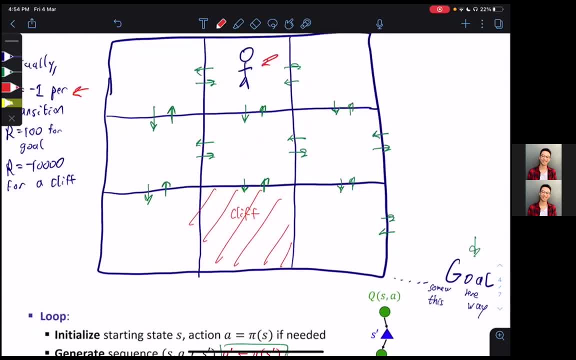 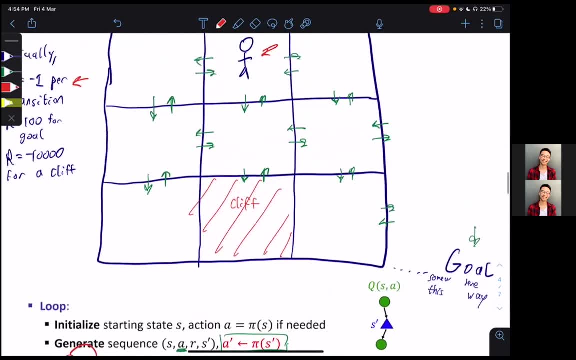 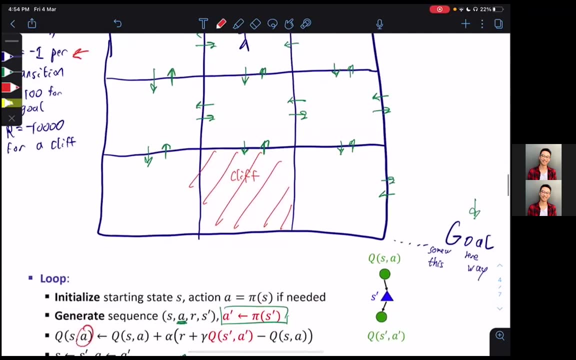 Okay. so right now we're over here, right? I'm going to walk through what SARSA does when it takes a step forward and generates the QSA value for this location, For this scenario right now, let's say our action for this state was to go downwards. I'm going to swap to my laser pointer. 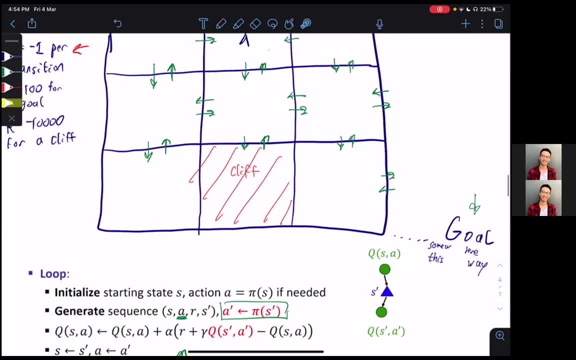 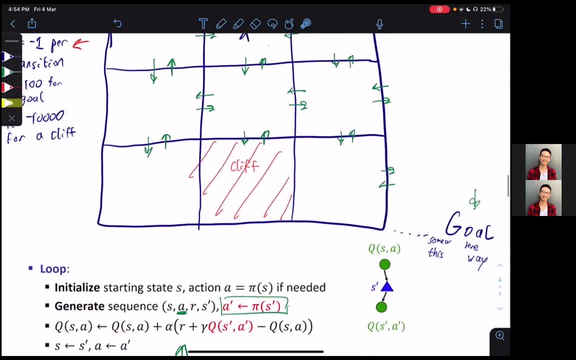 to go downwards. okay, This is done through this kind of generate sequence thing over here. Well, actually, technically, what happens is that the action was passed through from the previous iteration, but let's just say, like it's action right now for this current state is to go. 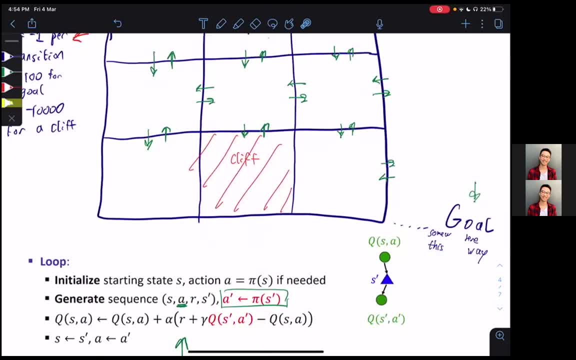 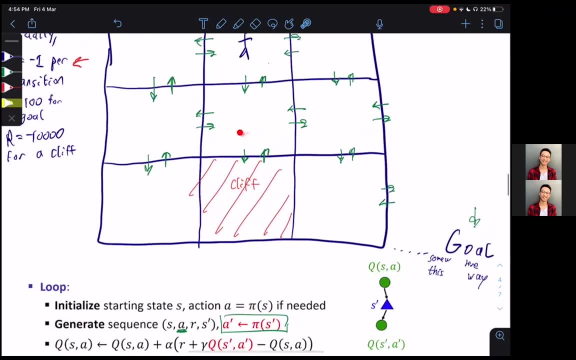 downwards. okay, But what's different about SARSA than Q-learning is that, in addition to generating the sequence and telling me where I'm going to end up- which is a S-prime over here? right, This is S-prime- I also generate the successor state's action. 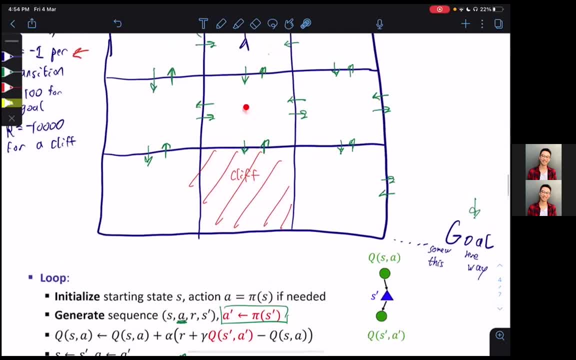 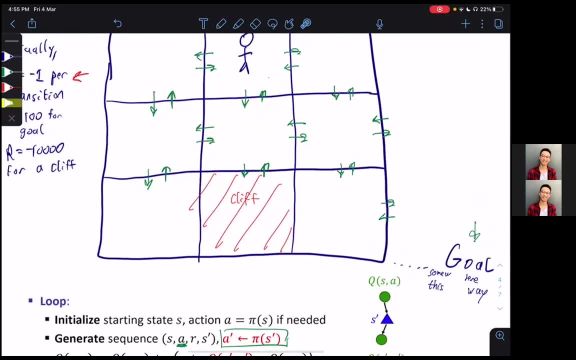 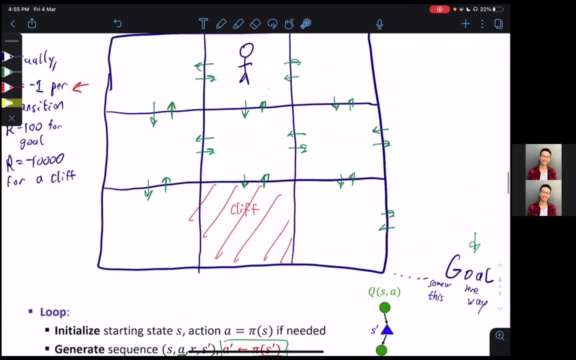 So A-prime. over here is some action from this cell right. So this is S, This is S-prime. A-prime is one of these green arrows over here which represent the successor state's action. So not only are we telling our program, okay, go forward one step, but also plan ahead one step. 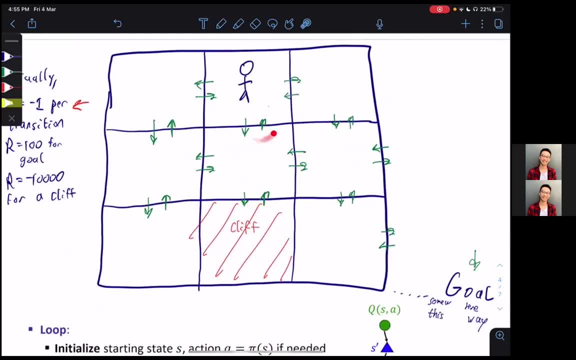 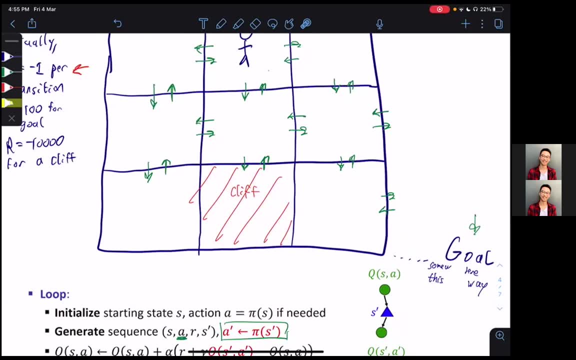 forward to go either here, here, here or back up, okay. So yeah, that's what we're doing. We're kind of thinking where Chris will be ahead by one step. So that's when we're just, I guess. 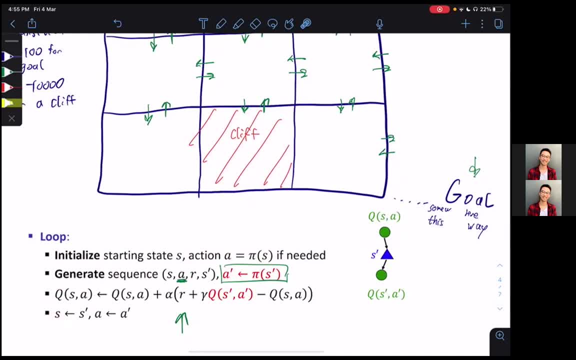 thinking and generating these actions. So now we're going to be updating our Q-value over here. So what happens over here? So this is simply, it's what it says. right, We're taking the Q-value of our successor state, this one and its successor action. let's say: 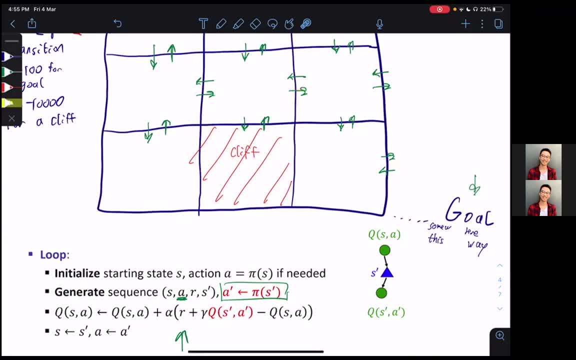 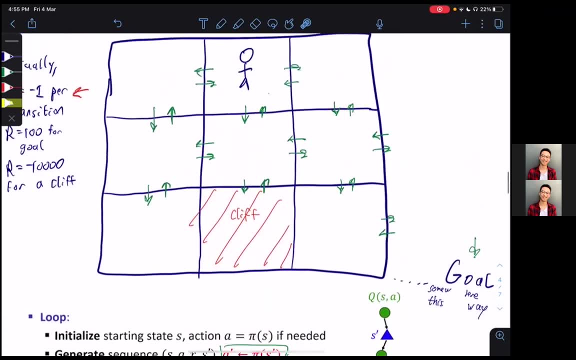 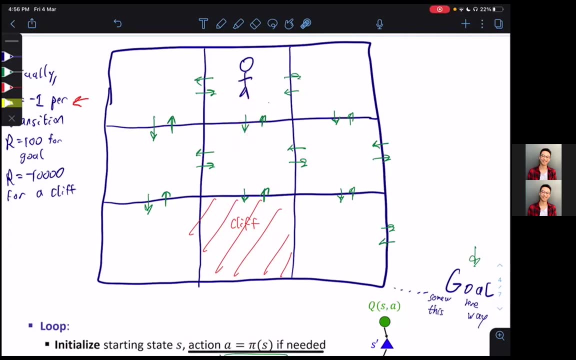 just we generate it to be this one right Minus Q-SA, which is our original state and our original action, right. So what this is saying is that when we're updating the utility of this state's, this action, so this state, and going downwards, we're updating this state and 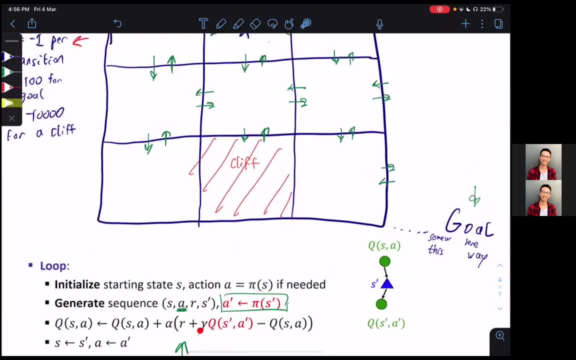 going downwards. we're also including, by some discount factor gamma, the utility of going to this state, of being in this state and taking this action. okay, So one more time when we're updating the utility of this direction, so this state going downwards. 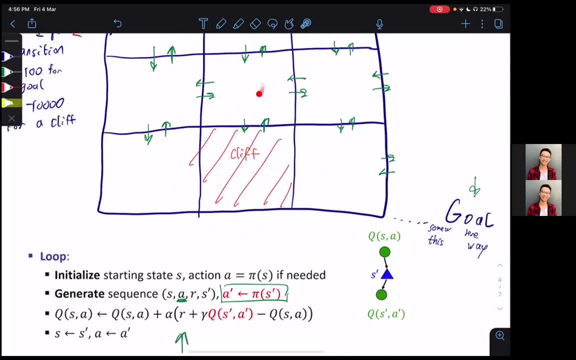 we're including the utility of being at this new state and taking this certain action. right, And you might be wondering: okay, how do we even generate this action in the first place? How do we choose this one? Well, all we chose or use was epsilon greedy. We use the epsilon greedy. 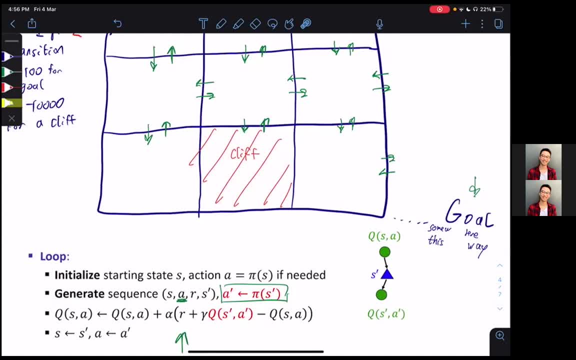 function to generate what actions best. So you guys might remember, epsilon greedy is a probabilistic function that chooses what actions it's best to generate. So that's a function that whether or not to exploit or explore by some- uh, probability epsilon right. so in some cases this 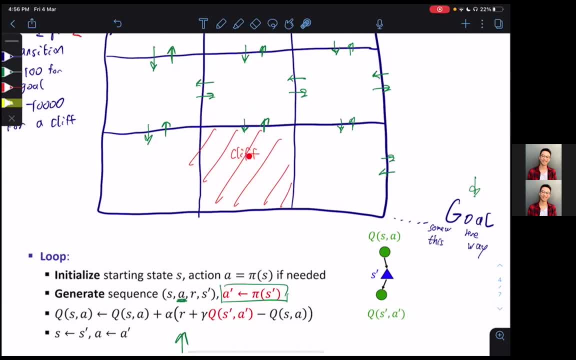 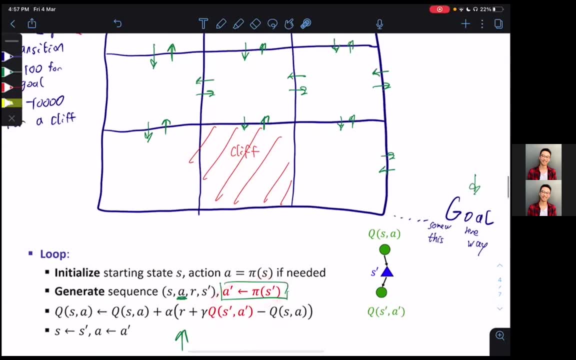 a prime could be telling me to go into the cliff, which is probably exploring, because this is. you know, why would i want to go here? this is definitely not right, but most of the time i'll be wanting to explore. so let's say, a prime told me to explore, uh sorry, most of the time i want to be exploiting. 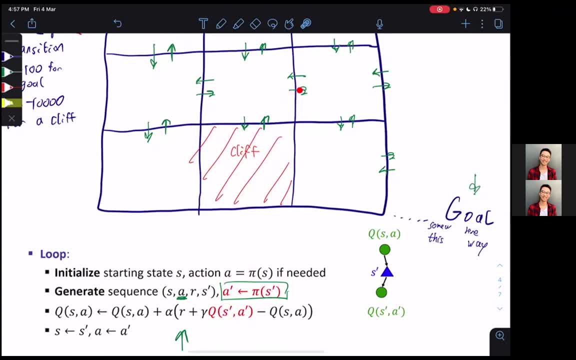 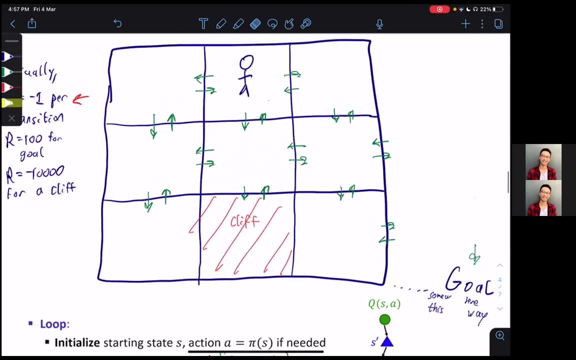 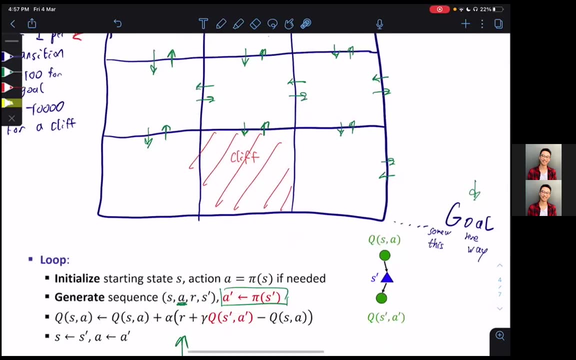 sorry, apologies, and a prime told me to go this way, so that's how it was generated. um one more and i guess, to wrap things up, when we're updating the key value of this state- oops, of this state- and going this direction, we also include by some discount factor gamma. 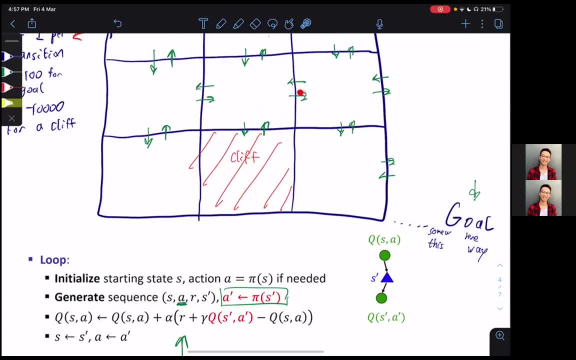 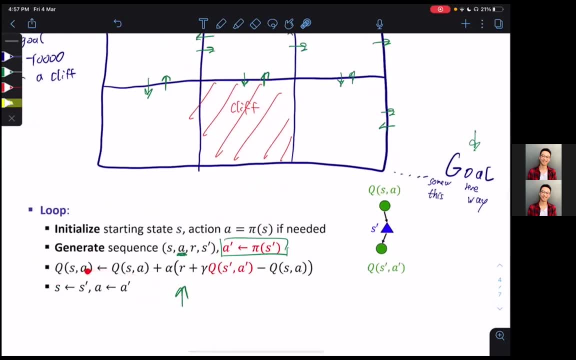 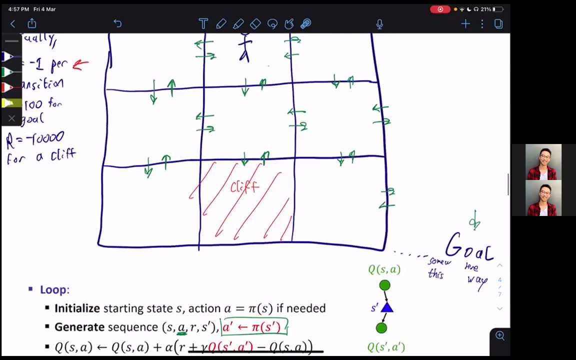 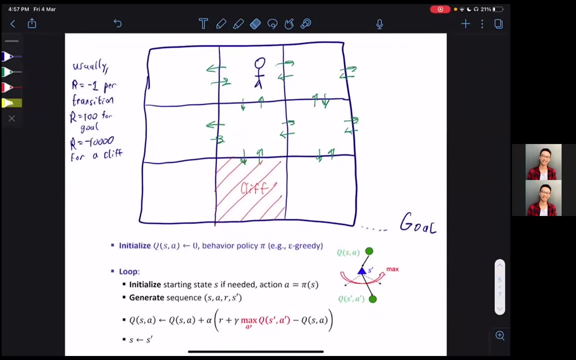 of that successor state and following that successor action, where we look ahead and we find that successor action using epsilon greeting, and then we pass that to the next state and we continue looking forward from over here. okay, so pretty simple, pretty intuitive. um, that makes sense. but what's different is that in q learning we don't actually do the exact same thing when we're. 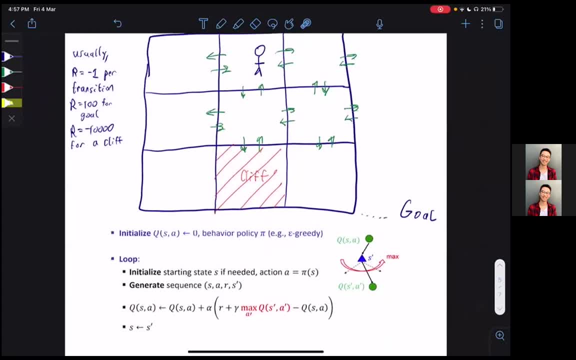 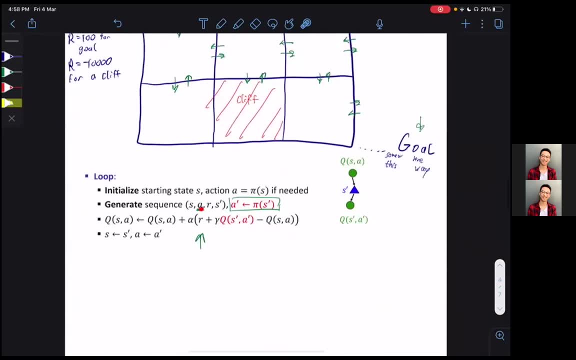 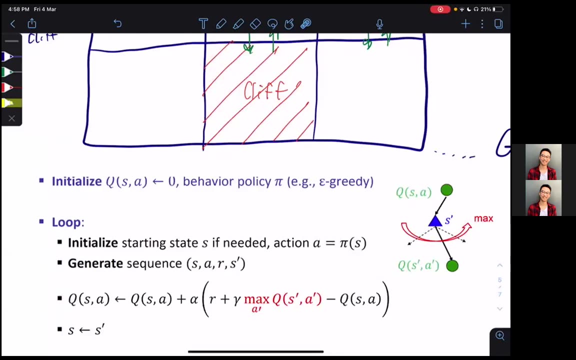 updating our key value right. so again, you can notice that we have this term over here and we also don't have an a over here. right before, sarsa spelled s-a-r-s-a, sarsa right, but here we only have sars, so it was the same right. this is saying that we don't generate a prime right. all we do from this. 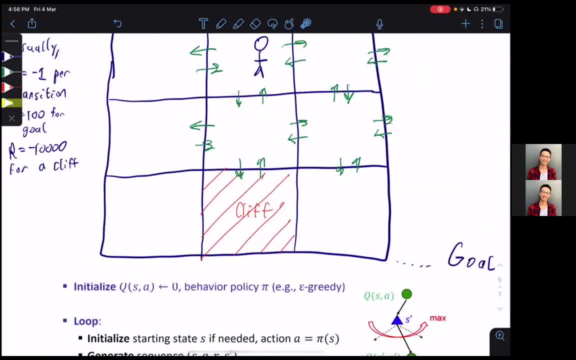 state is that we know that we're going in this direction over here, but we don't generate or look ahead and say, okay, i know i'm going to be taking we don't. we don't call epsilon gritty on this state and say, okay, i'm gonna go here or here or here, we don't know yet right, we just say, okay, i'm gonna. 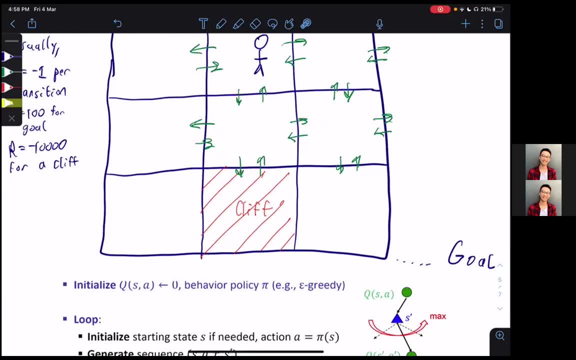 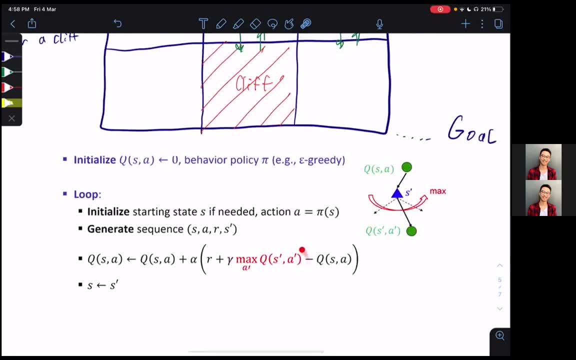 tell myself i'm gonna be going in this direction first. right, pretty simple, makes sense. but the difference is when we're updating our q value, right? so what happens? we're updating our q value, we run this instead: max Q S, prime, A prime. So all we're actually doing over here is saying that, okay. 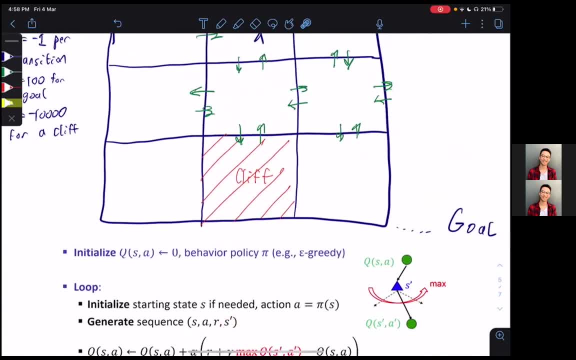 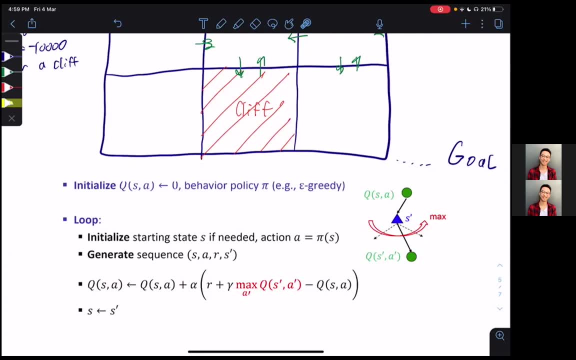 I know I'm going to end up over here, right. I know I'm going to end up in this S prime over here right Now. forcefully tell me what's the best and most optimal action in this S prime over here. 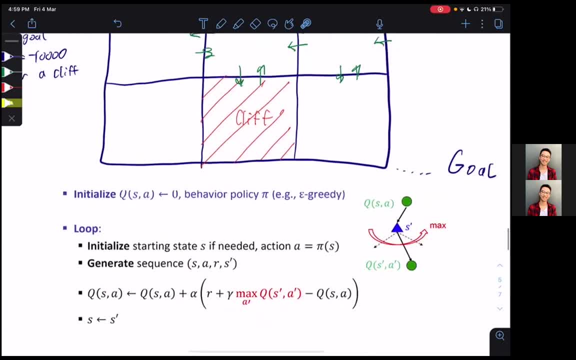 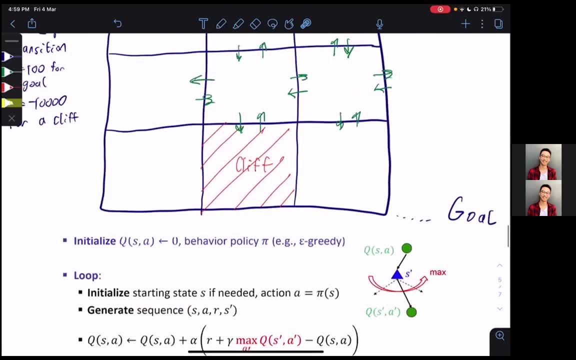 right, And in this case, this best possible action is probably going in this direction or something, because the goal is over here, right? So we probably want to go in this direction, right? So when we're updating our QSA value for this state, when we update our QSA value, 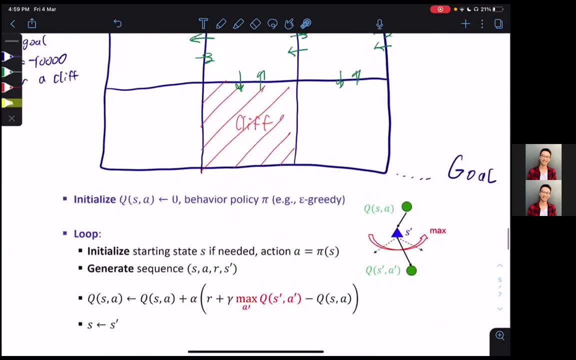 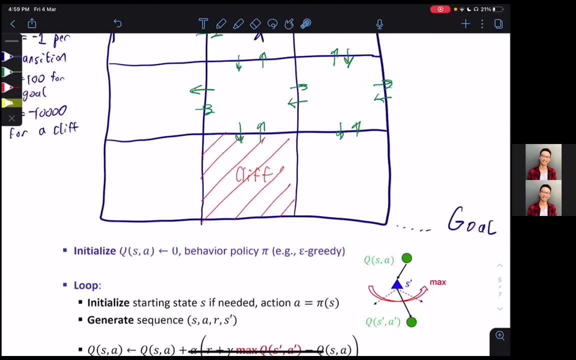 we include the action or the utility of going in this direction, which is this QS over here, but we also include the most optimal action possible, even if we don't decide to go there, which is this one. So you might be thinking, okay, you just demonstrated the exact same thing. 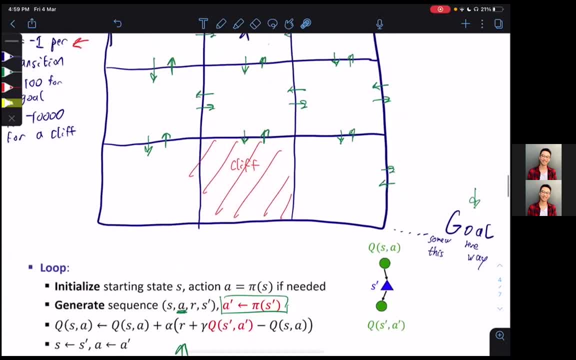 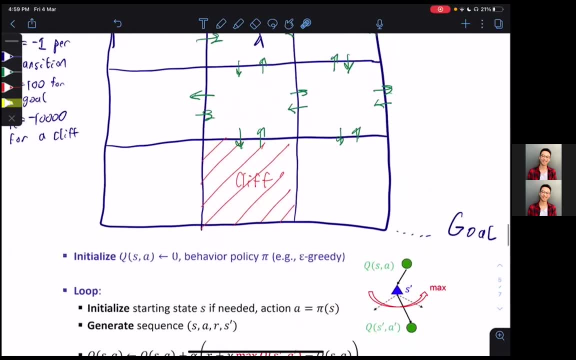 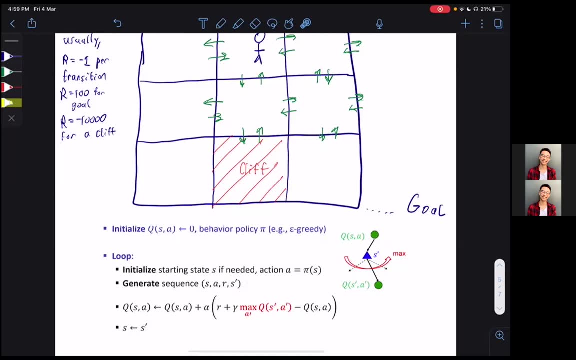 right Over here. A prime told us to go over here and A told us to go over here. Same with Q learning. how is this any different? right, Well, it's different because, remember, we're not actually generating and telling ourselves to do A prime. right, Look over here. right, It says A equals. 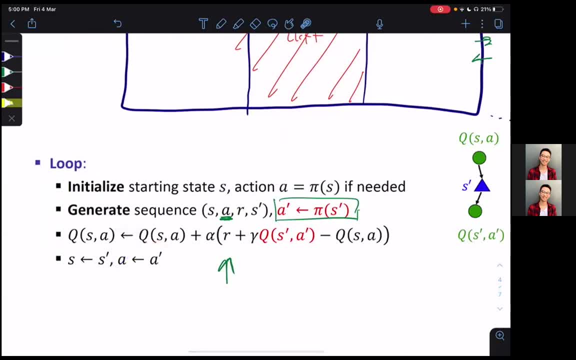 A prime. Oops, sorry, A equals A prime. right, I actually follow through with my promise I made over here. I made a promise that at the successor state I will go through with A prime and I'll update with A prime and I'll actually go through with A. 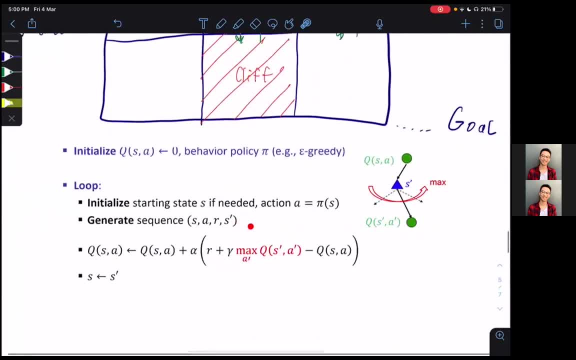 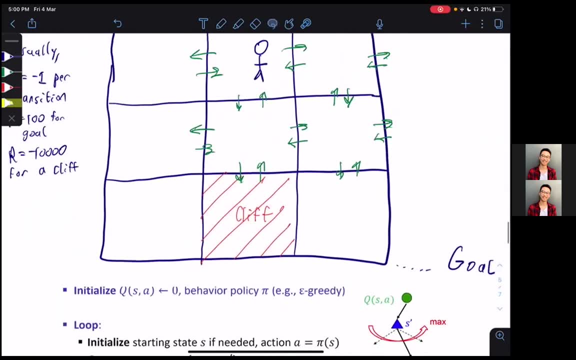 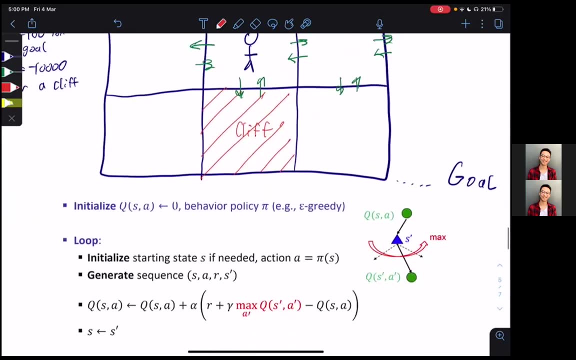 prime. But in Q learning I don't have that promise. I don't actually tell myself that I'm going to follow through with A prime. So what does this mean? This means that, okay, let's say, I'm at QSA, I run the algorithm, I move my guy over here, right, because we follow action A and then we run. 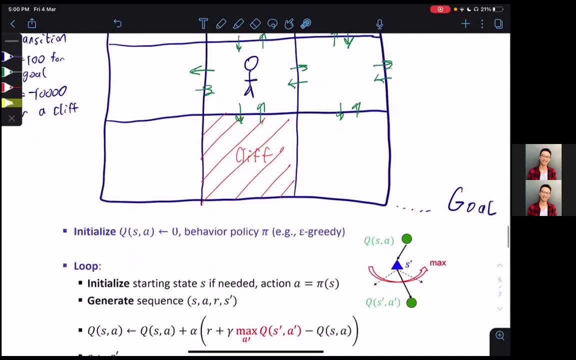 generate sequence SARS, right, But then, at this state, my A could be in this direction, right, I could choose to explore this, right? So I'm going to go through with A prime and I'll update with A prime. So I'm going to go through with A prime and I'll update with A prime. right, So I'm going to. 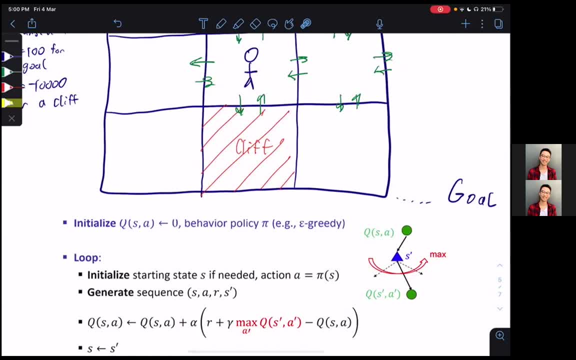 run Epsilon gritty for this state Right now. this is S. We're not at S prime anymore. This is S. now right Action can tell me to go over here. But what's different is that remember when we were back over here in the previous iteration, when we were back over here in the 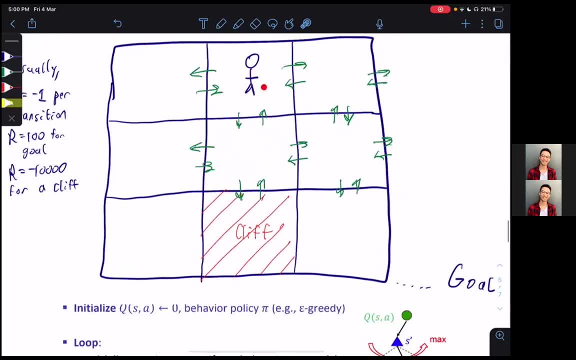 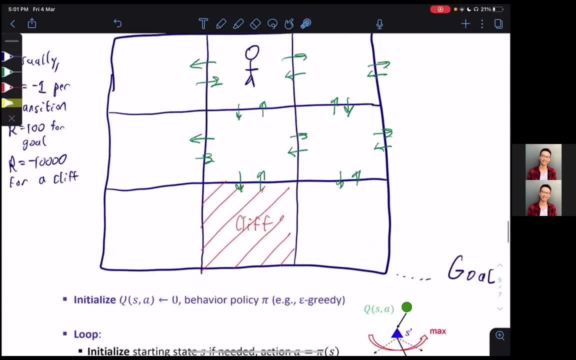 previous iteration we updated this Q value with this action- not over here, right? Because we just assumed that, oh, when we're over here, we're probably going to go over here. So I'm just going and promise and assume that we'll always take the optimal action at each successor state. 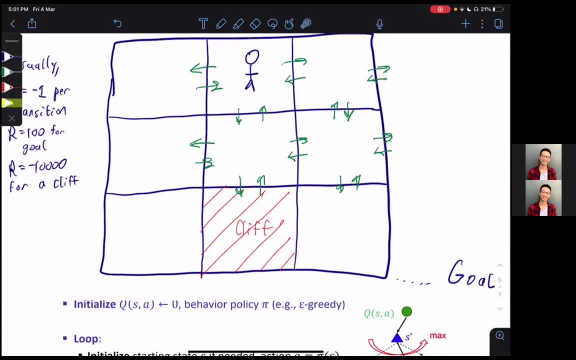 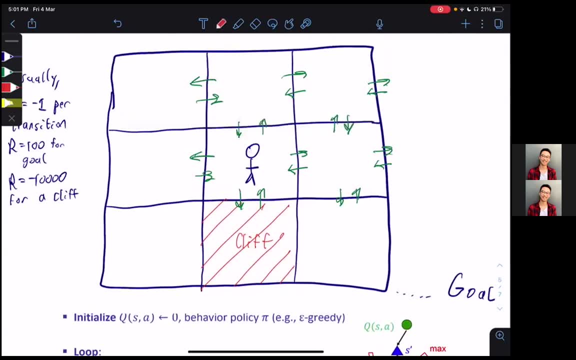 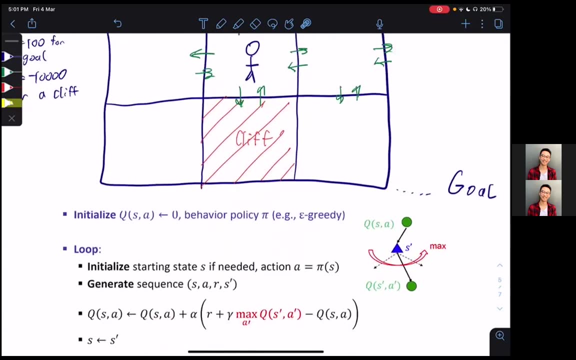 So the Q value for this, the Q value for this action, was updated using the most optimal action, But when we actually ended up going over here- right, We actually ended up going over here and generated an action- We ended up choosing an action- QSA- that is actually in this direction. 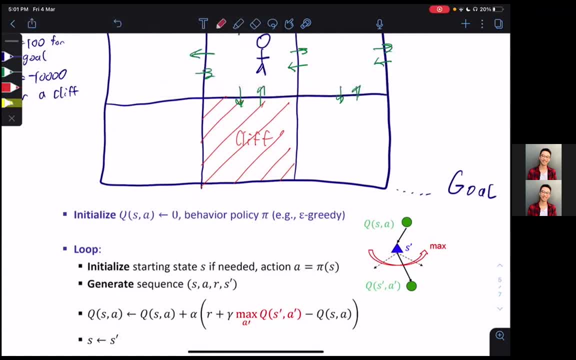 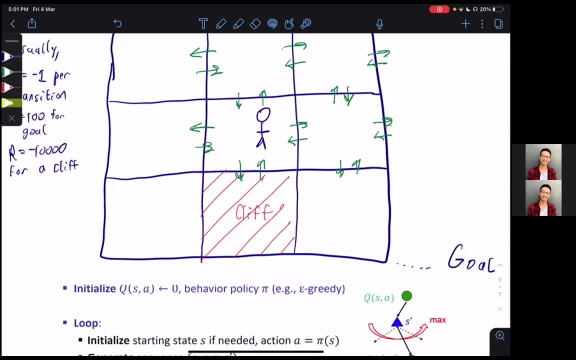 And we ended up ending up over here later, right? So that's pretty interesting, Right? Because when we're- when the robot was exploring and trying to figure out where to go right, It ends up doing a path that goes something like this, right, Like that, But when it was over, 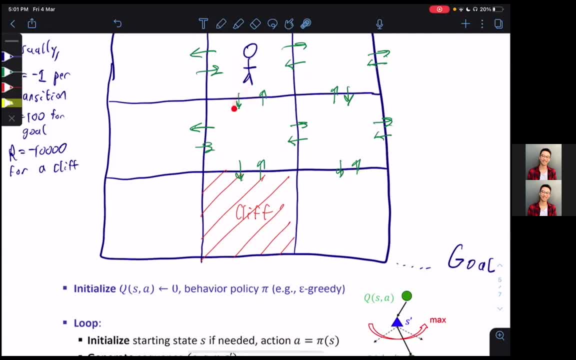 here and updating the Q value for this guy over here, which is the down direction which we all decided on. it was updated by assuming that we'd always take the optimal path, But in reality that doesn't always happen, And sometimes I might even slip into a cliff, right, So that's. 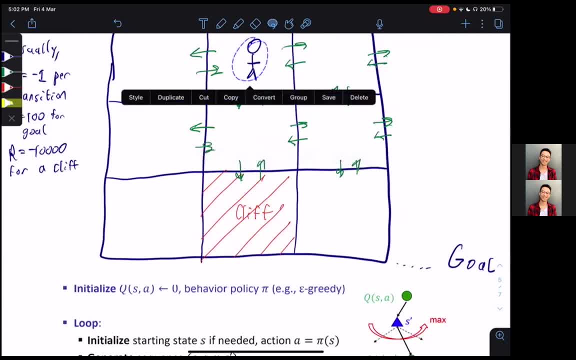 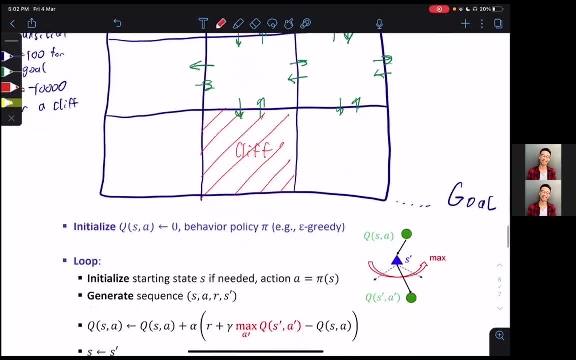 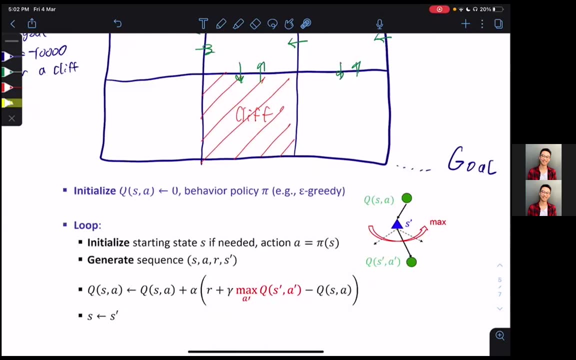 that's kind of messed up right. It assumes that I'm always going to take the optimal path, but that's not always going to happen because, remember, I could always slip, I could explore something. So that's why I guess Q learning is often known as the very greedy algorithm. It's not. it's not realistic. 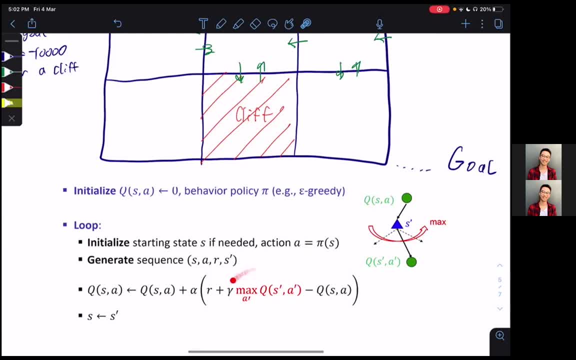 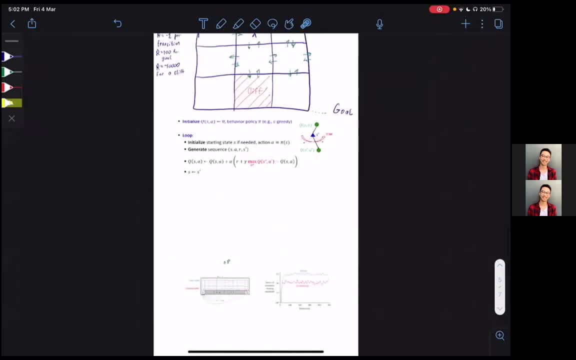 right It's. it just assumes that the successor action will always be the most optimal. So hopefully that makes some sense. I'm going to be applying another example down below, which I think will hopefully explain more things. This is a more generalized- and I guess we're not generalized, but like a more 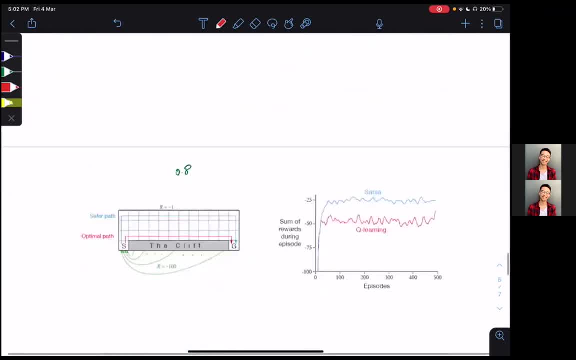 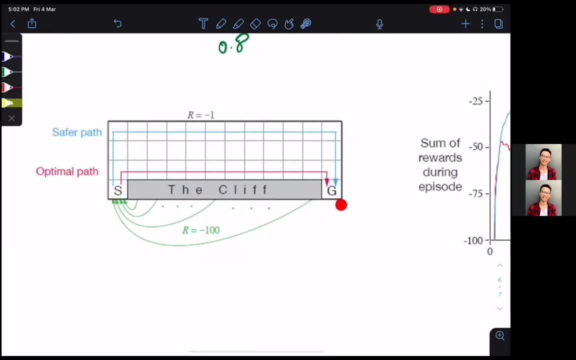 I guess bigger version of this grid role over here, right? Let's say we're starting at this goal state over here and our goal at the start state and our goal is to get to this goal state over here. right, When we run Q learning in Sarsa, it's going to spit out a bunch of Q values that. 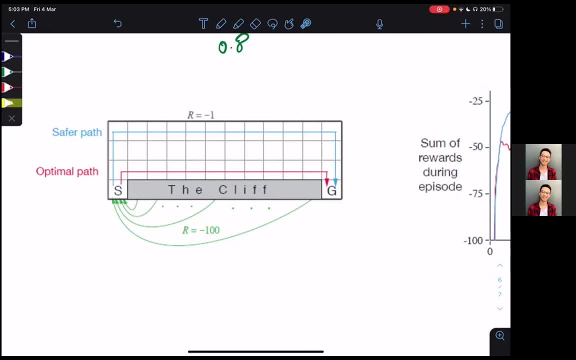 will give us a policy, a bunch of optimal policies that will tell us the optimal path of the goal. Q learning tells us that the optimal path is this way. Sarsa tells us that it's this way. So notice something here, right. 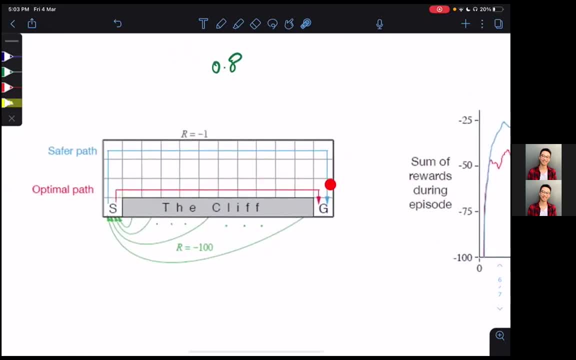 The Q learning path is much more optimal, right, but it's also much more unsafe, right. The safer path is not optimal, but it's a lot more safe, right. Okay, I mean I, I know I just reused the same word, but like, do you get my point? Like, 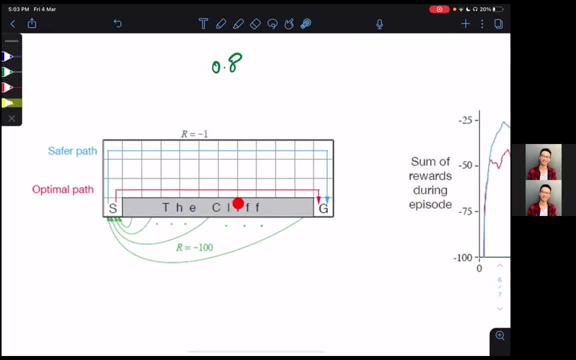 like this is much faster, but it doesn't come from the fact that I might fall into the cliff. Now let's think about why. doesn't it count for the fact that I fall into the cliff, Like I could just easily fall and slip into here, right? 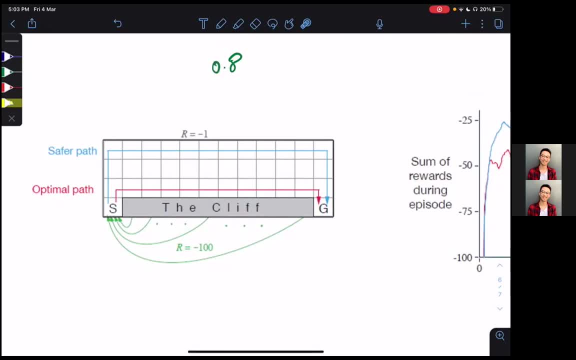 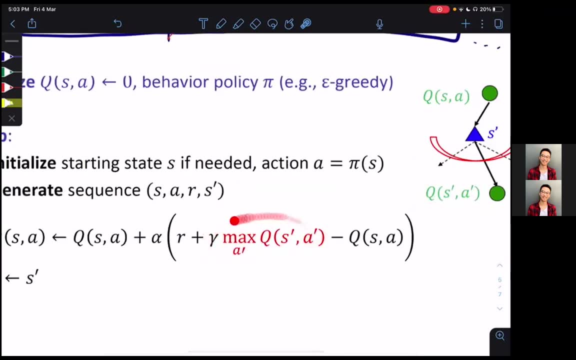 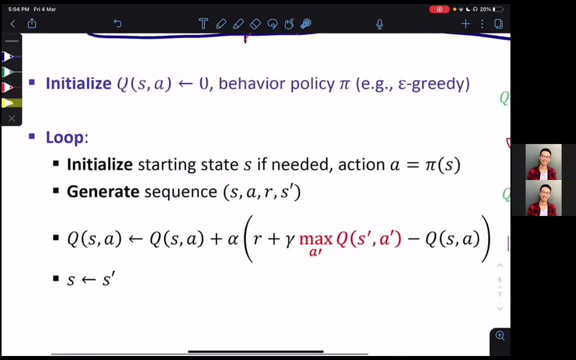 I could you know? transition probability is like 0.8 or something, right. I could easily fall into the cliff over here if I slip. Why doesn't it count for that? Because it's optimistic right When in the beginning, when it was generating all of its Q values. each Q value it generates, right is done by calculating the optimistic successor state action pair. 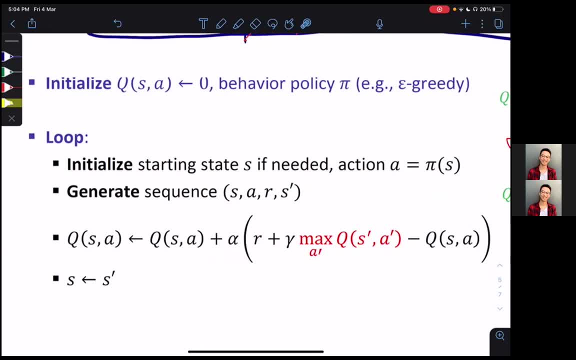 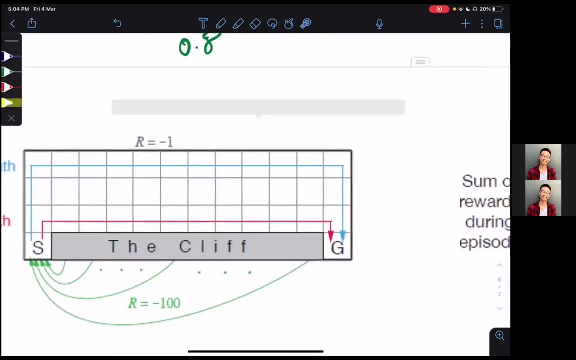 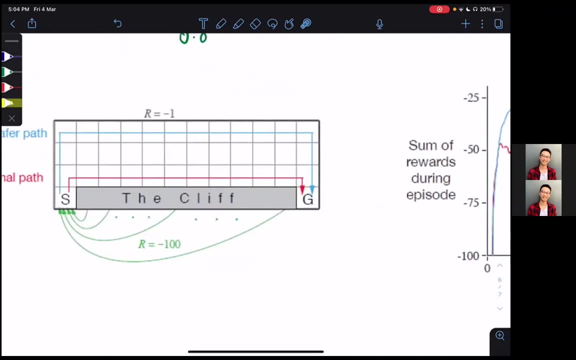 The optimistic successor state action pair. Because it's optimistic, it doesn't account for the, I guess, utility of potentially falling into here. right, Obviously the Q values that are closer to the goal will have higher utility, right, Because you know it's closer to the goal, right? 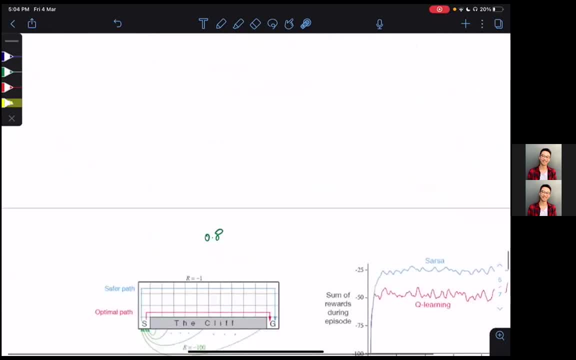 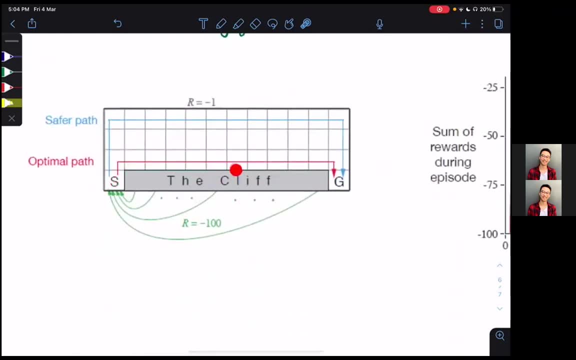 And if it doesn't count for the fact that I might slip and fall to the cliff or just do something wrong. that's why it doesn't really care. It doesn't care about this, like this chance of falling into here, Because when the Q values were being generated, it just assumed that we're always going to go this way, right. 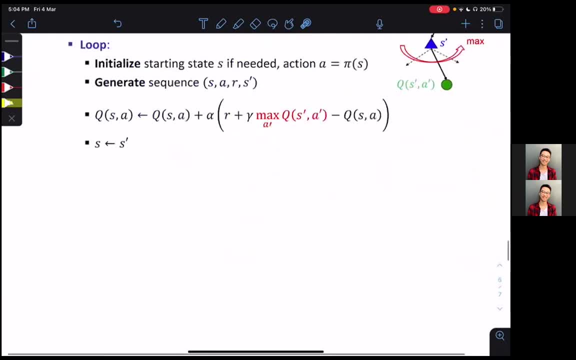 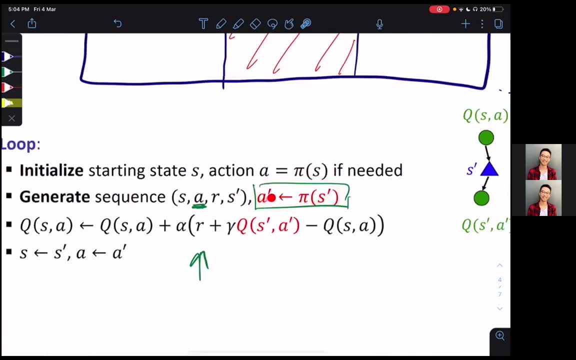 Because of this max over here. But for SARSA- remember SARSA- when we call generate sequence, we make a promise. We make a promise that we'll actually follow through with the successor state action. right, That's why we have A equals, A prime over here. 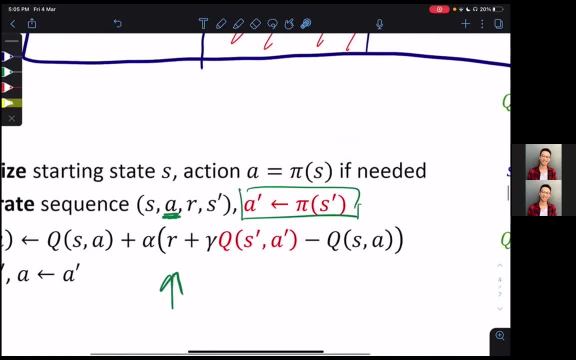 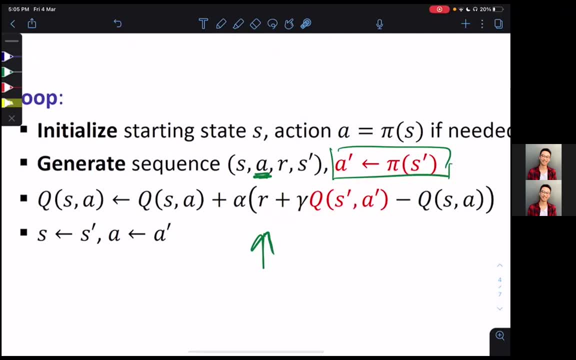 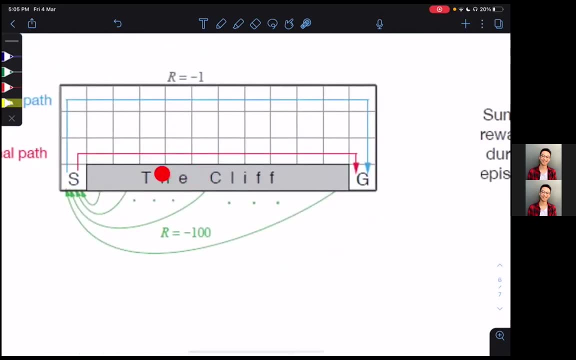 And because we make this promise and use that, we use this promise to update our corresponding Q value right. We use this promise, this promise right, To update our corresponding Q value right. The chances of potentially even falling into the cliff over here and dying are a lot higher, right. 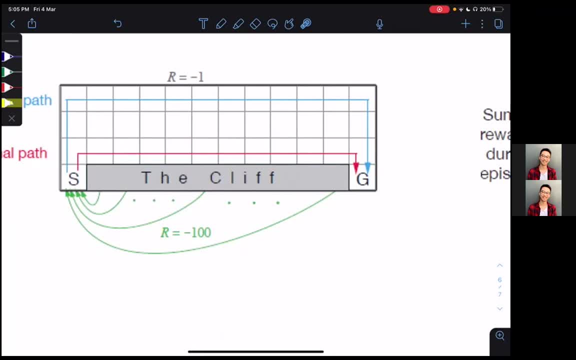 Oh no, no, sorry, not the chances, but like they account for it more. It's the same chance of falling and slipping to the cliff, But the chances of that actually happening are just more accounted for because it falls through with that promise. 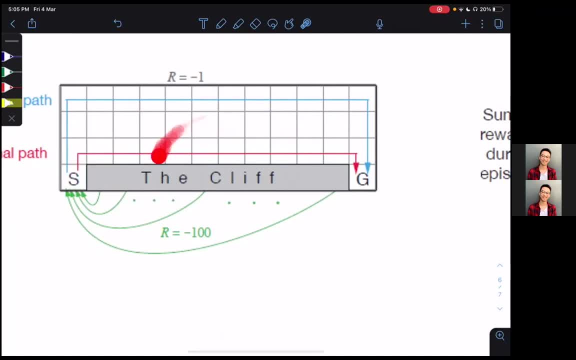 So when the algorithm is running through this entire thing, right, going wherever all the place, and for the time to like over here and like over here and falls into a cliff, right, The Q values account for that, And they get scared like, oh crap, I don't want to be over here, right. 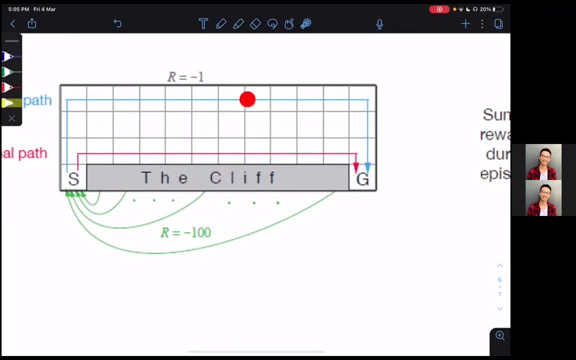 Last time I was over here, I fell into the cliff, So I'm going to stay over here. I'm going to put more utility for these values and these policies And when I'm over here, I'm going to tell myself to go up.